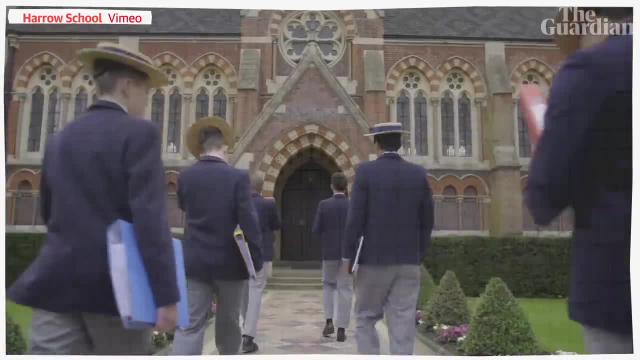 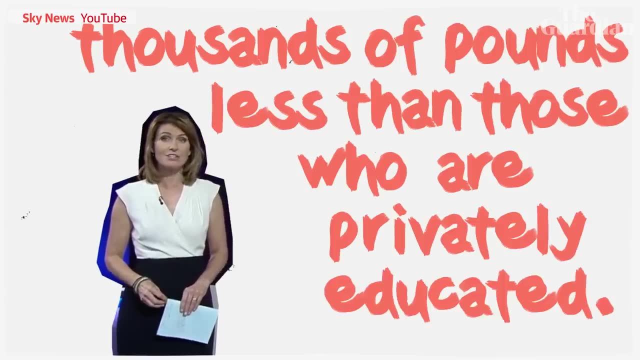 The thing that is most distorting our education system is the existence of private schools. State school graduates are still likely to earn thousands of pounds less than those who are privately educated. What we're seeing is entrenched privilege. Why are the people at the top? why are they ever? 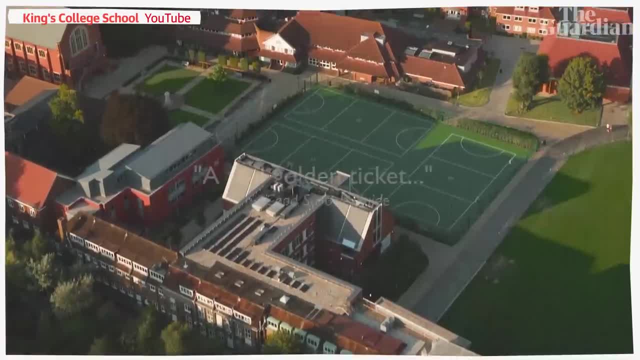 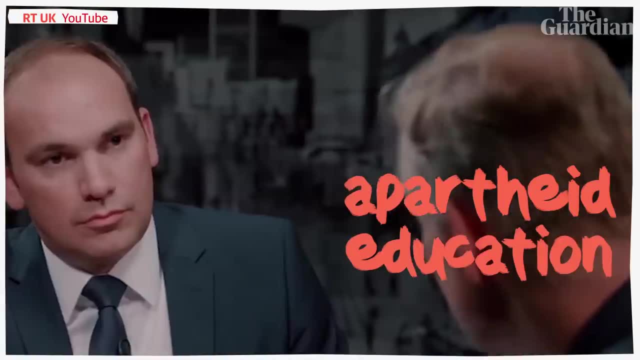 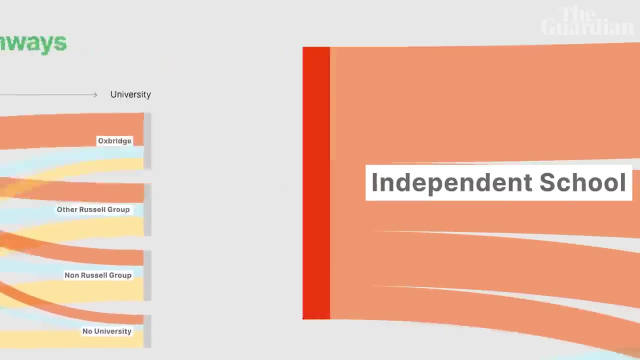 going to want people like you or I taking the jobs that they want to go to their privately educated sons and daughters. We will have an apartheid education system in this country unless we do something drastic. There's an endless stream of evidence that private schools help make our 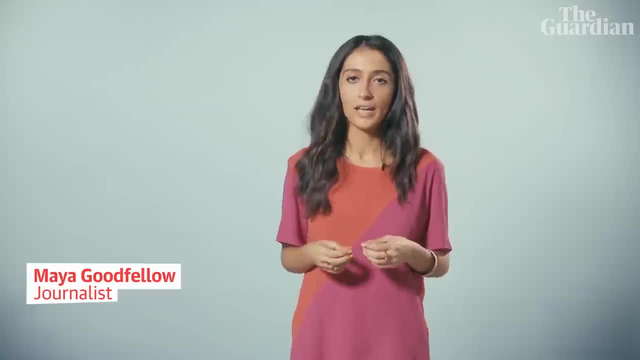 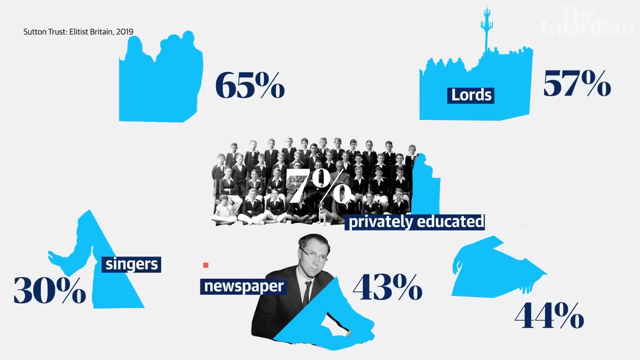 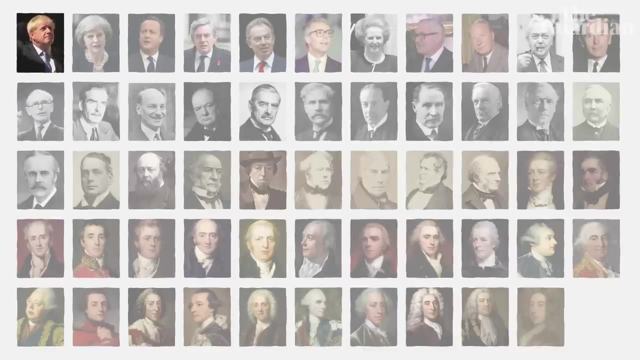 country unequal. Only seven percent of the UK are privately educated, but a disproportionate number occupy some of the most influential jobs, whether in media, art, law or politics. I mean, take our new prime minister, the 20th to be educated at one school, Eton. 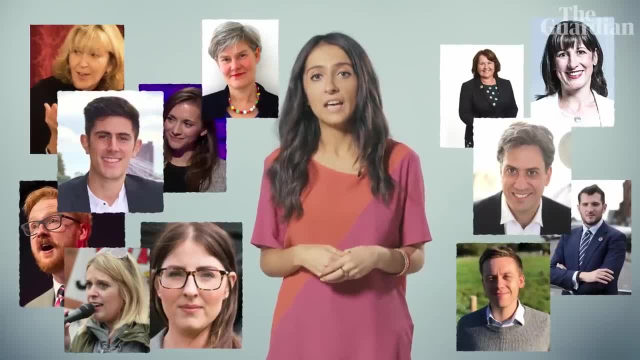 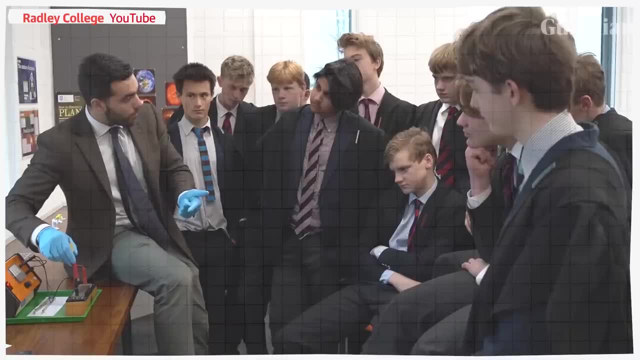 But now a number of people are asking if this is fair and if they should exist At all. As a state school teacher, why would I not want the absolute best for the young people in front of me? Why don't they deserve to have small class sizes, luxurious facilities, access? 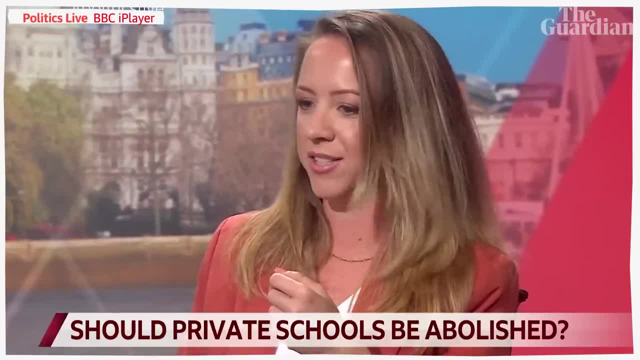 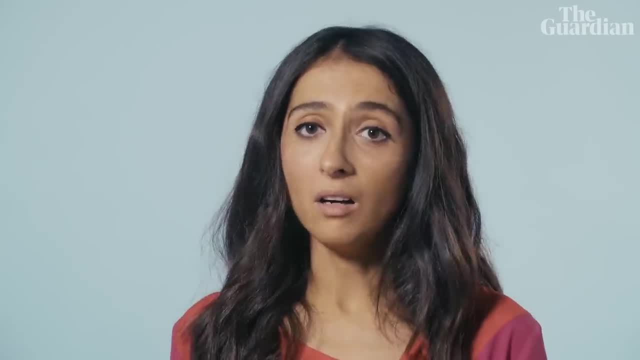 to this incredible network of alumni and I think that would make our society much better and much fairer, and abolishing private schools is key to that. But before getting to abolition, we need to know what private schools are and how they work. Well, the origins of Britain's private schools. 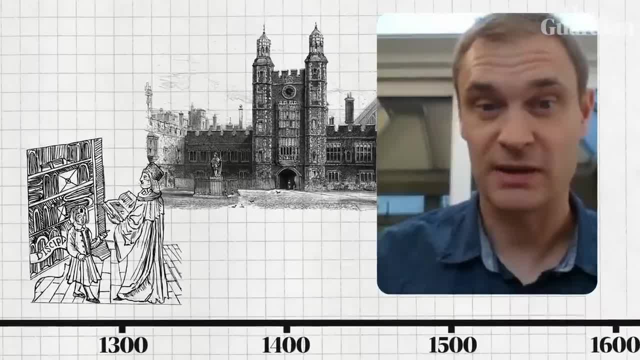 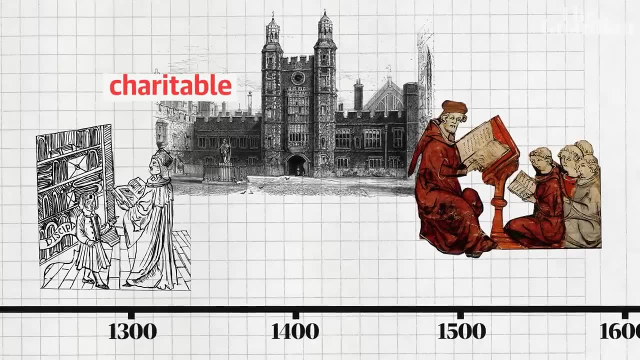 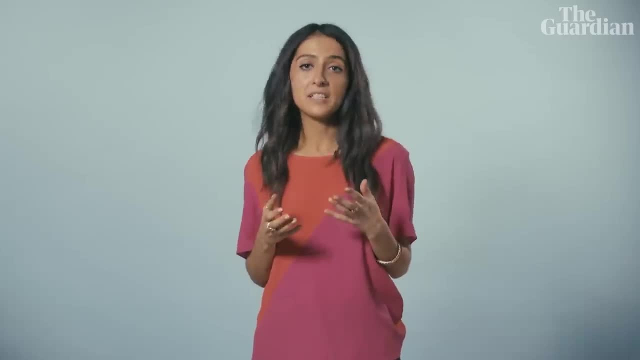 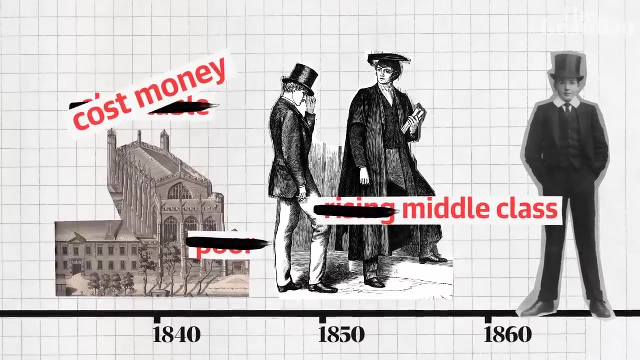 date back into the medieval period, the late medieval period, with a series of charitable bequests to educate the children of poor and rising middle class families. So they started out as charities but gradually they expanded in the Victorian era when they became increasingly for the middle classes and they cost money. This trend continued into the 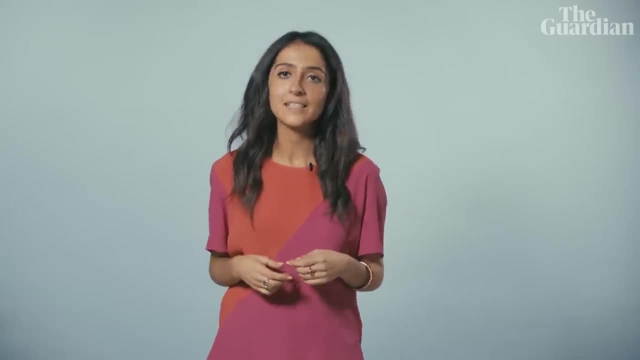 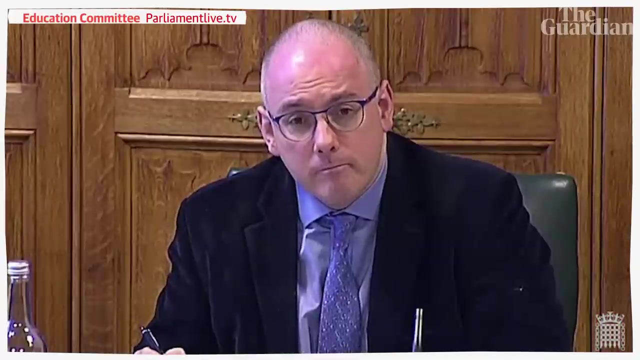 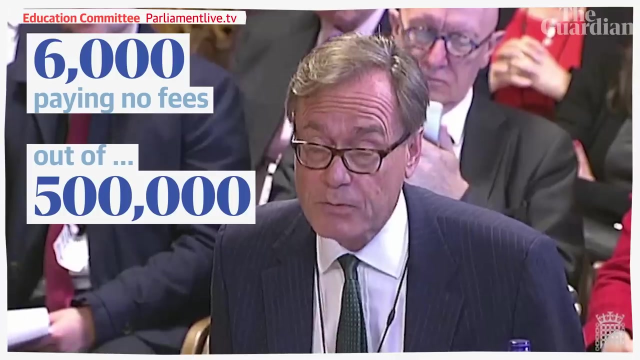 20th century and to avoid being labelled elitist, in the 1960s they re-branded as independent schools. Fast forward to now, And how inclusive are they? So that's 6,000 pupils paying no fees at all out of the 1.5 million pupils in independent. 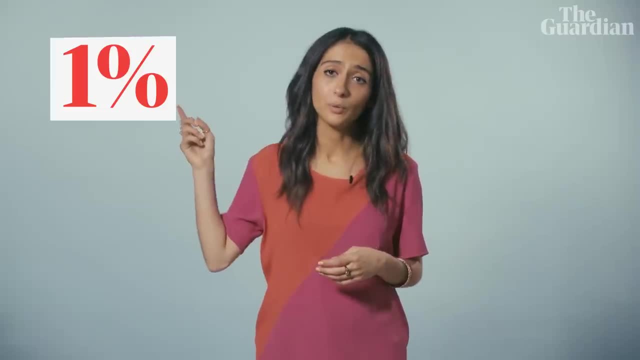 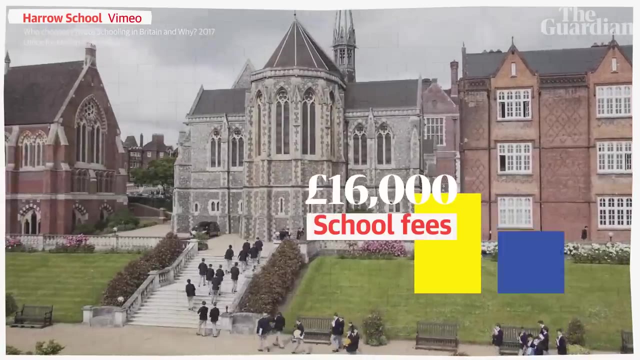 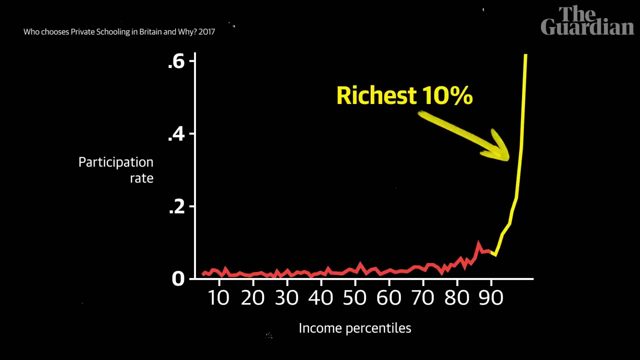 council schools. Turns out, that means only one percent of people who go to private school are from the most disadvantaged backgrounds. But most people can't afford to go private. Rising school fees amount to 50% of an average earners wage, which is why intakes are dominated by the very wealthy. So, while funding has been cut by the current fiscal year, school fives are less than 50 per cent of social care. So, while funding has been cut by the coming fiscal year, the average salary is around £5 per cent in the 20th century. 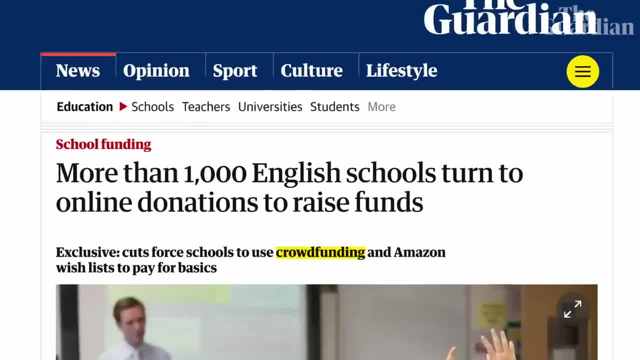 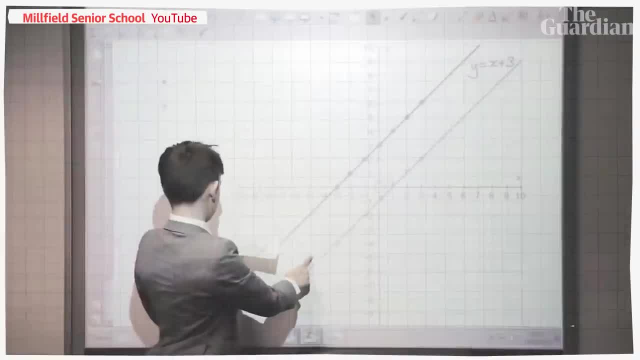 Which is why the income increases of the migrant population is becoming more and more significant, cut to the point that state schools are having to use crowdfunding and amazon wish lists to pay for basics. a tiny proportion of people get access to the excellent support and almost unlimited. 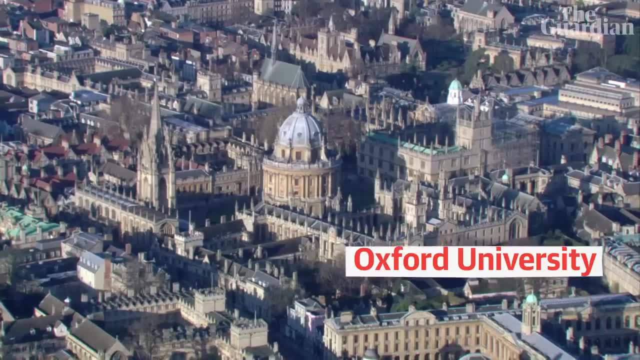 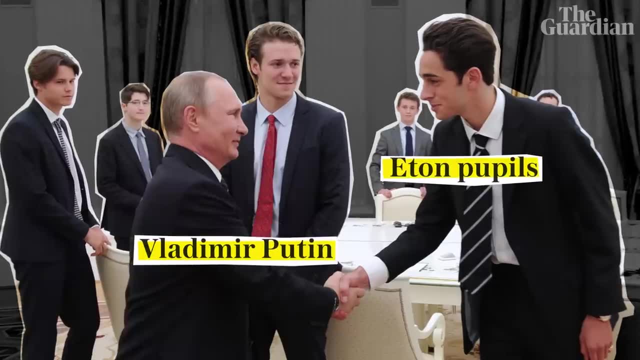 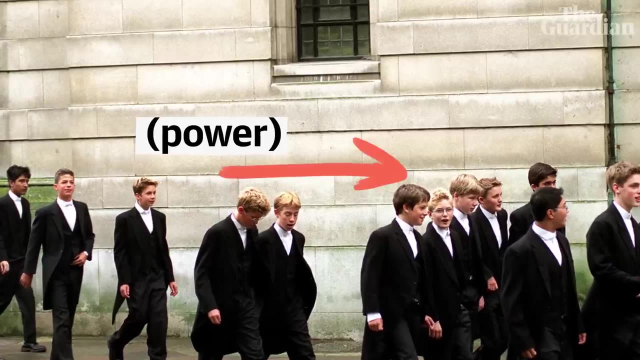 resources that the private sector offers. plus, private schools act as a direct route to prestigious universities and networks, to some of the world's most powerful people. but discussing what to do about private schools isn't about attacking the choices that parents make. it's about an elite system that fast tracks certain children. so what can we do about this? 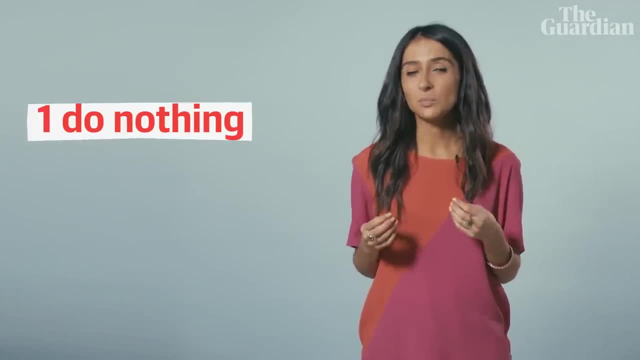 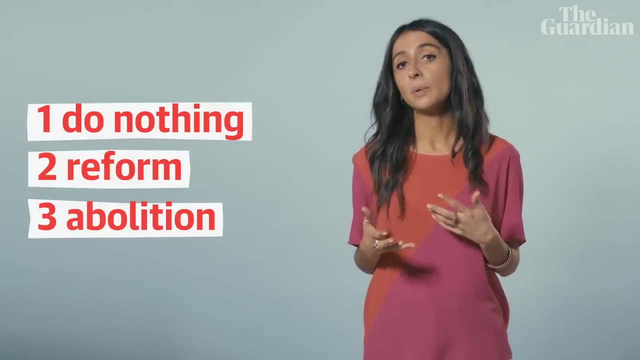 broadly, there's a few options. we could do nothing, which means there's no point watching this video. we could reform the system to try and make it fairer, or we could get rid of fee-paying schools altogether. let's look at reform first, and the main point here is: although they mostly 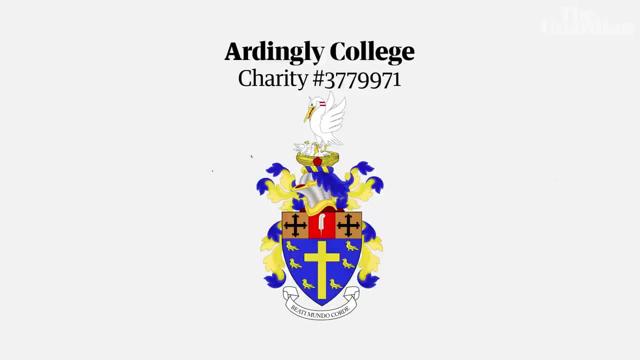 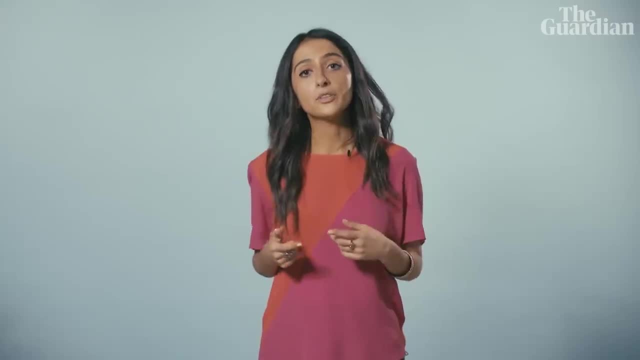 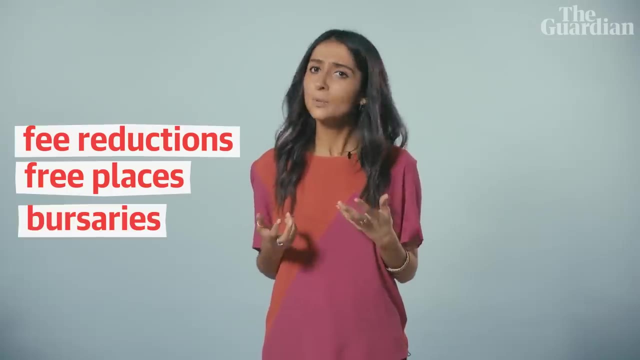 educate the well-off. over half of all private schools still operate as charities today. has there ever been a more deserving charity? many private schools say they earn their charitable status by offering fee reductions or free places in the form of bursaries. so a simple measure could. 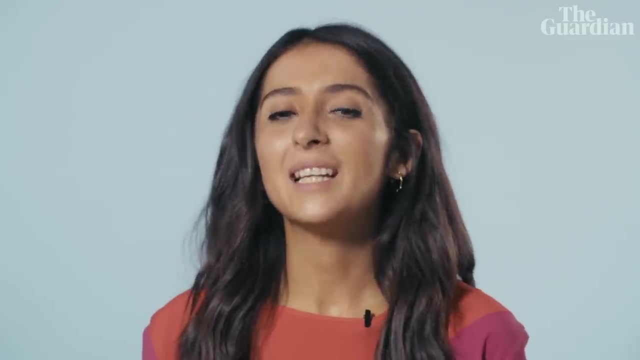 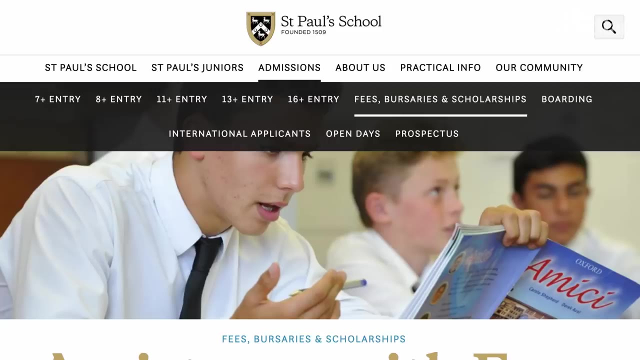 be to demand that they offer more, but that would still only be a limited number of people, and these bursaries are often used to top up fees of people who are already pretty wealthy. we even found one school willing to offer financial help to families so long as they earn less than 120 000 pounds. also as charities. private schools don't pay full business rates, so getting them to pay the full whack- which is something state schools already have to do- could bring in an extra 105 million pounds per year. another idea could be to charge vat on private school fees. 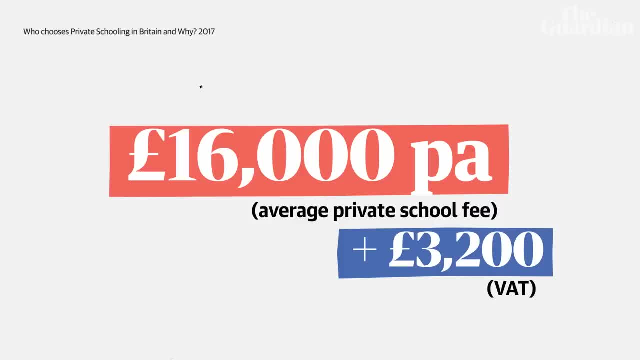 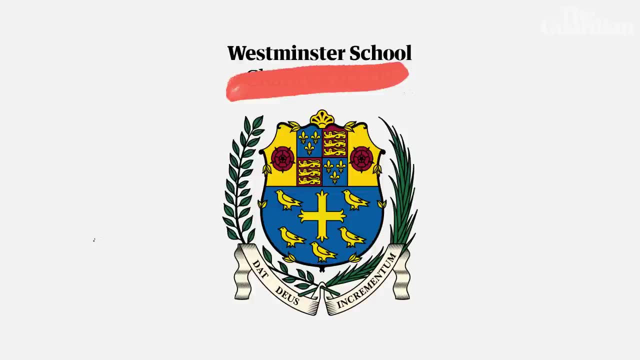 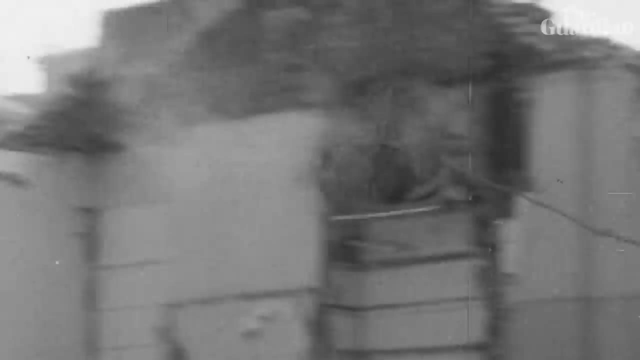 since they're currently exempt. that could bring in an extra 1.5 billion to the treasury, or you could just strip them of their charitable status entirely. but what about something? you're not the only one who can do that. well, there are even bigger, like abolition. 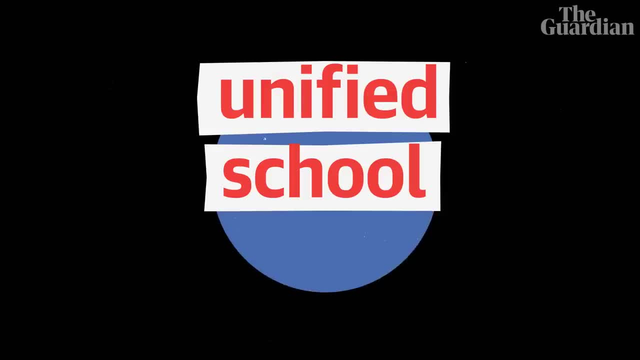 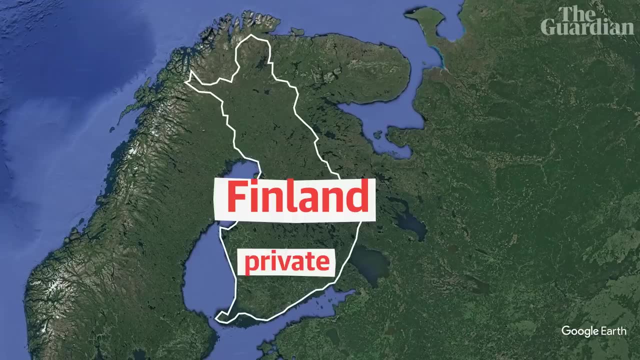 look, let's not get too dramatic here, because the idea of abolition isn't about destruction. it's about unifying and integrating our education system. that's what they did in finland. their education system used to be a mix of private grammar and state schools, not so different from ours, but in the 1970s the government has done something.